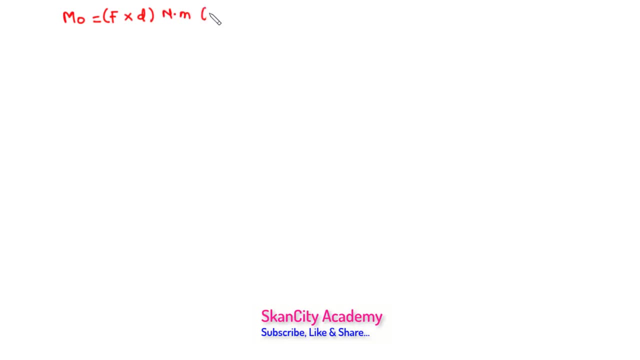 is measured in Newton meter. Now, in today's video, we are going to learn how to find the moment of a force in three dimension. Now, in three dimension, it is very difficult to obtain the perpendicular distance, and so we are going to use a different approach or method, that is, the cross product. 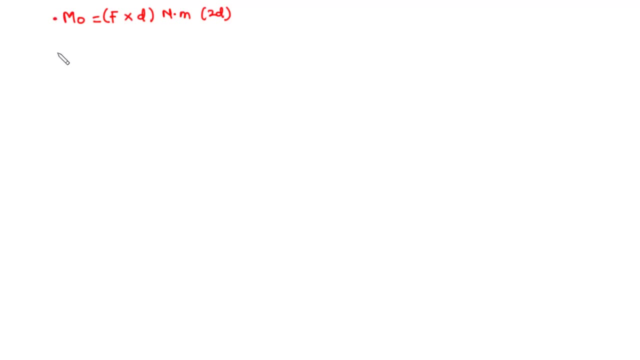 multiplication. So, in three dimension, the moment of a force is given by the cross product of r and then f, where r is said to be the position vector, the position vector directed from O to any point on the line of action of f, and then f is said to be the force represented as a Cartesian. 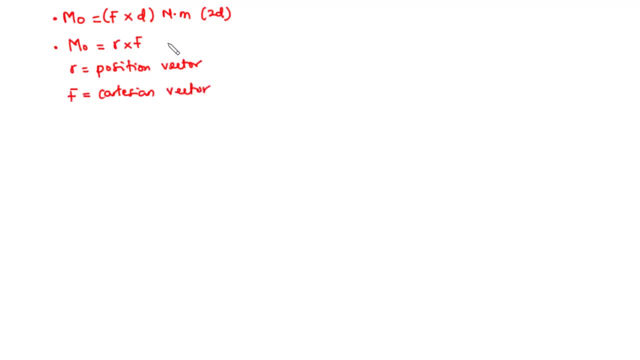 vector, and so the moment of a force in three dimension is given by the cross product of the position vector directed from O to any point on the line of action of f, and then the force, f represented as a Cartesian vector. Now let's assume that we have a force. 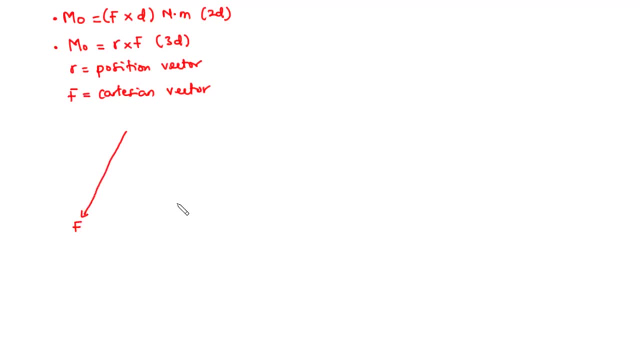 acting along this line. and then we have a point O where we are going to take the moment about. Now, the first thing we are going to do is to specify a position vector directed from O to any point on the line of action of f, and so we are going to treat this. 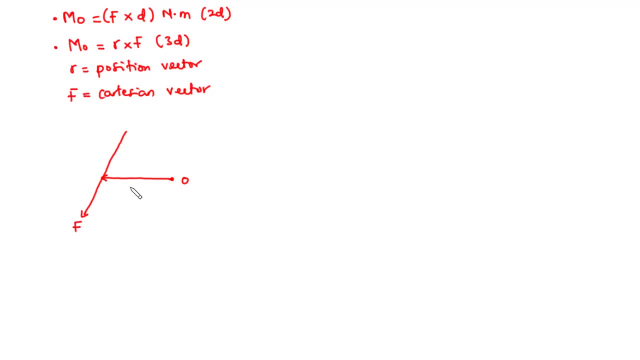 position vector as a sliding vector. Now you realize that this R is not perpendicular to the line of action of F, and so we define some distance, say D, which is perpendicular to the line of action of F, and then we also say that let the angle formed between R and then the line of action of F on this side 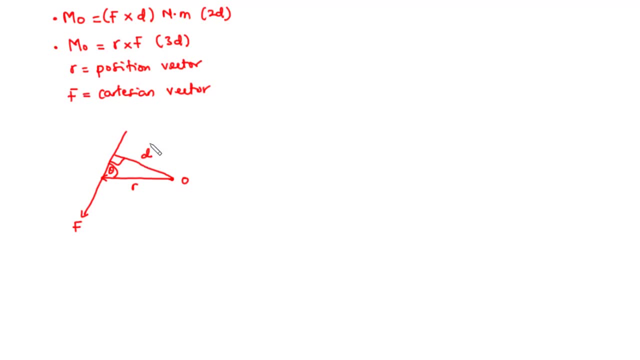 be theta. Now, in that case, then we have the perpendicular distance, D to be equal to…. since this angle is facing this side, then we say that D is equal to R times sine of the angle theta. and so, since we have the perpendicular distance and the magnitude of the force, then we say that the moment about 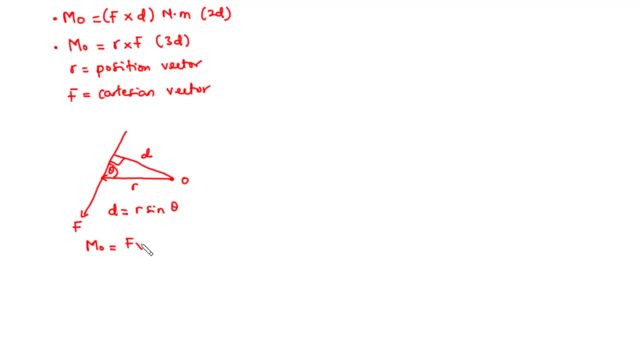 the point O is giving us the force times the perpendicular distance. We have perpendicular distance to be r sine theta, so we have r sine theta times f, and that is equal to r f sine theta. so this is the moment of the force. and then we have the moment acting vertically. 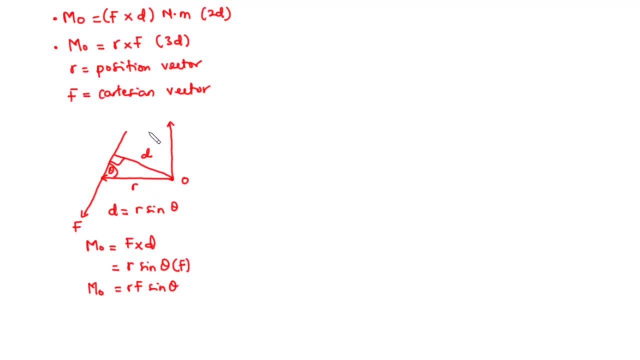 upwards at O. so this is the moment at O. Now talking about the direction of the moment, the direction of the moment can be obtained by considering or applying the right hand rule. so let's assume that this is the right hand. so we have the fingers and then we have the thumb, which is acting vertically upwards, or? 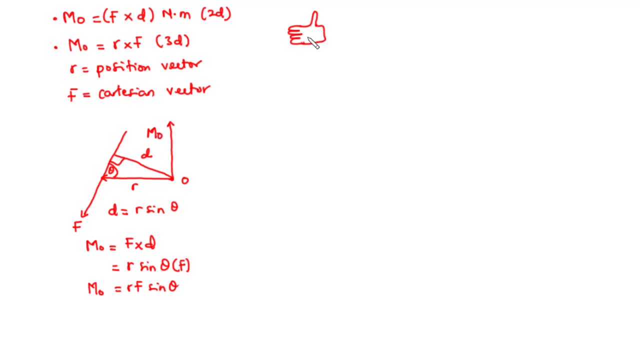 acting perpendicular to the plane containing r and then f. Now, if you want to kill the fingers of the right hand, you realize that you are going to move in the anticlockwise direction, that is, you move from r towards f, and so you realize that the moment is in the anticlockwise. 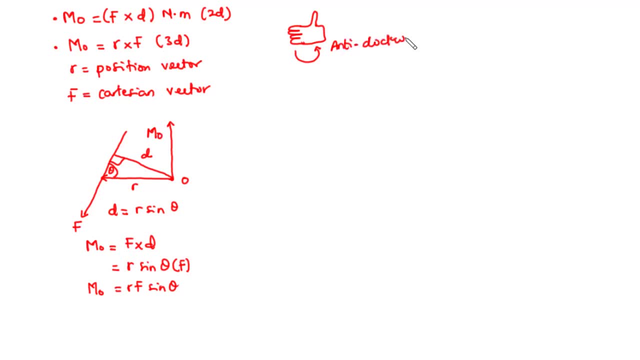 direction. So the moment about the point O, which is giving us the cross product of r and then f, has a direction which is in the anticlockwise way. Now, one important thing you need to take notice of is the fact that cross product is not commutative, that is, r cross, f is not equal to f cross. 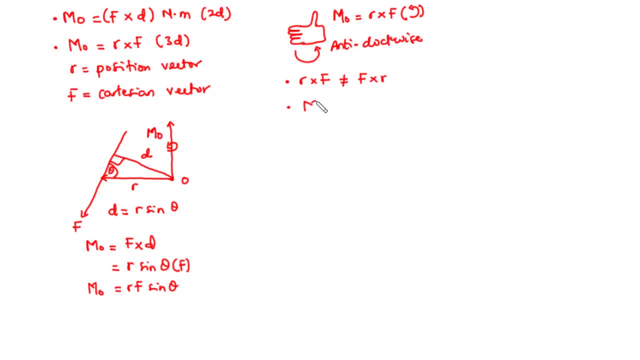 r. therefore, the right order of the moment of the force, which is given as r cross f, should be maintained in order to obtain the right sense. So, basically, this is the formula we are going to use to find the moment of a force in three-dimension as far as cross product multiplication is concerned. 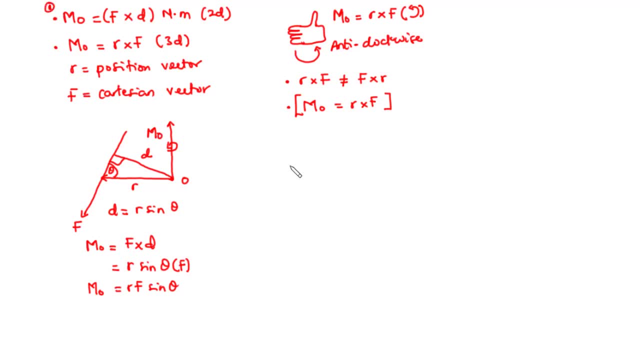 Now let's move on to the second item we want to discuss. So, secondly, if a force is acting along this line, Let's say we have a force which is acting along this line, the force F, and then we have this to be point O, And at point O this force is acting on this line. 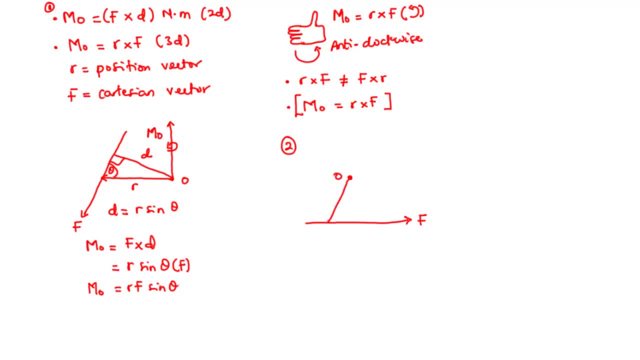 So if the force Directed from O to any point on the line of action of F, we have the position vectors R1, R2, and then R3. And then let's assume that we have the moment acting vertically upwards here. Now, according to the principle of transmissibility, if you have more than one position vectors directed from O to any point on the line of action of F, 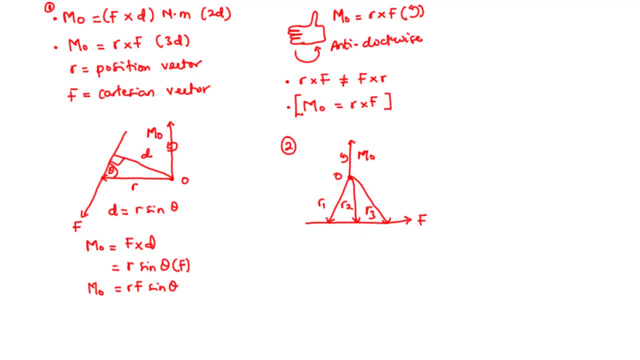 then the same moment will be produced at point O, if you want to consider each of the position vectors. So what we are saying is that, given If you have more than one position vectors, if you want to find the moment of the force about the point O. 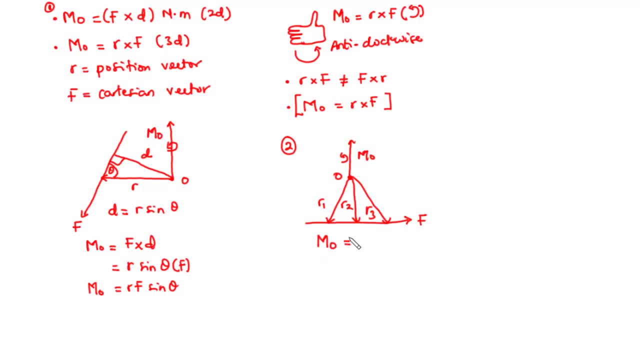 then it is basically giving us You can have the cross product of any of the position vectors and the force and you are going to obtain the same moment. So MO is equal to. You can choose R1 cross F and that will be the same as R2 cross F. 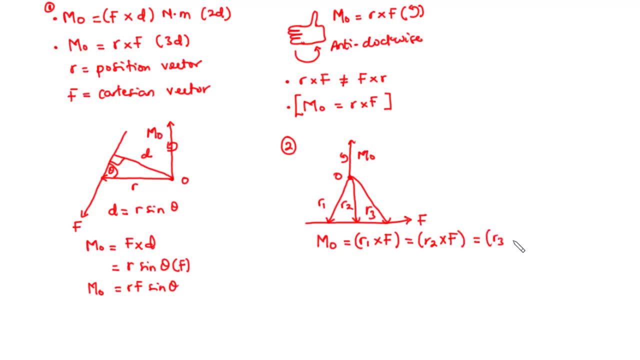 And that will also be the same as R3 cross F. So whichever position vector you consider, be it R1,, R2, and then R3,, the cross product of any of these position vectors and F will produce the same moment. 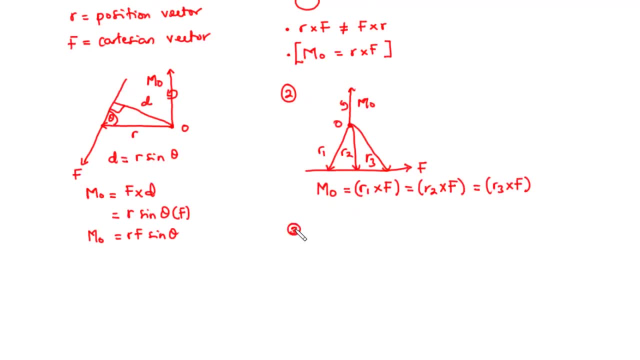 Lastly, if a body is acted upon by a system of forces and then you want to find the resultant moment, the resultant moment of the forces can be determined by the vector addition of the moment of each of the forces. So let's assume that we have this to be the XYZ plane. 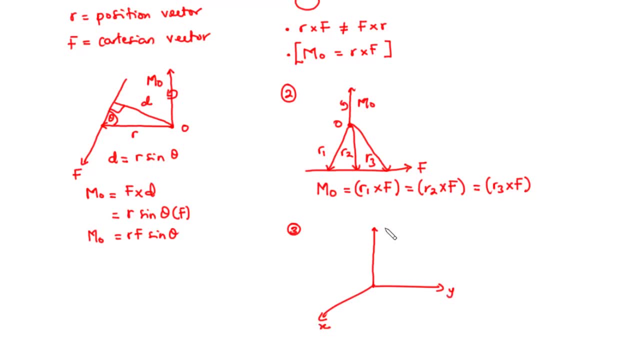 So this is the X-axis, Y-axis, and then the Z-axis, And then we have a body which is acted upon by a system of forces. So we have this to be F1.. We have, We have F2, and then this is F3.. 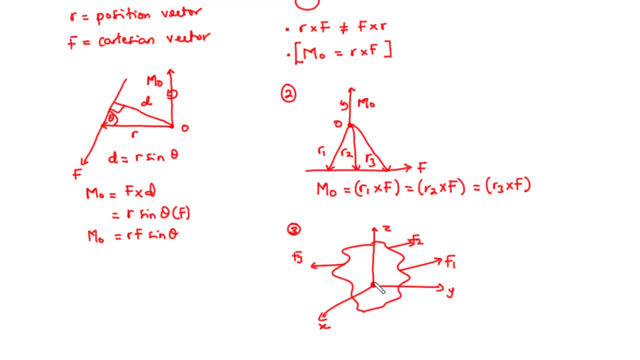 We also have a point O, and then we have the position vectors directed from O to F1, F2, and then F3.. So these are R1, R2, and then R3.. Now, if you want to find the resultant moment, 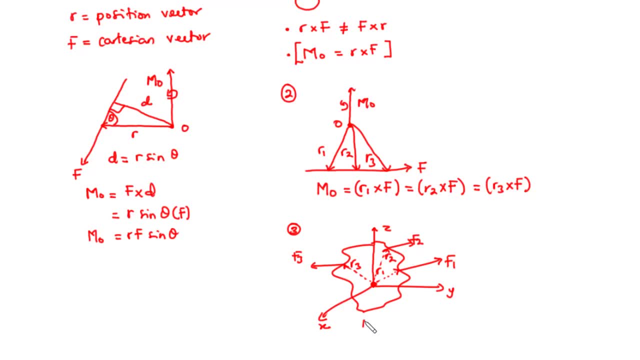 acting on this body, then we say that the resultant moment is equal to the vector addition of the moment of each of the forces, And so we have the cross product of R1, and then F1, plus the cross product of R2, and then F2,. 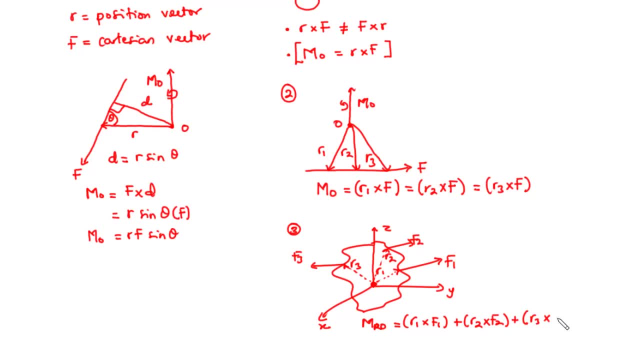 plus the cross product of R3, and then F3.. So basically, the resultant moment acting on the body is given as the summation of the position vector R times the force F represented as a Cartesian vector. Now let's kindly take notice of the fact that 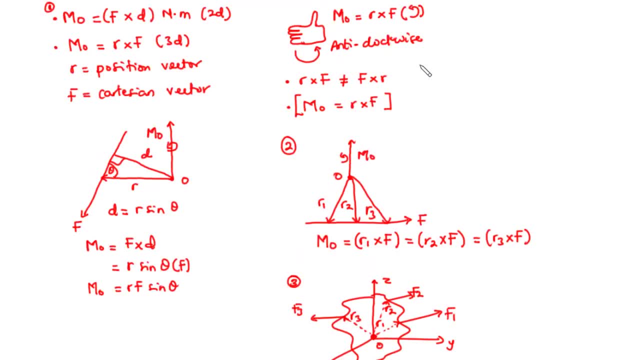 moment does not always act in the anticlockwise direction. Now let's assume that we have the right hand and position such that we have these to be the forefingers and then we have the thumb vertically downwards, or acting vertically downwards. 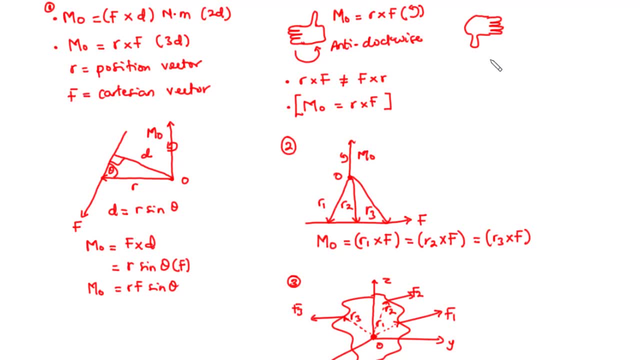 Now, if you want to find the moment of a force or to take the moment, you realize that if you curl the fingers of the right hand, it's going to move in the clockwise direction. So this time we have the direction to be clockwise. 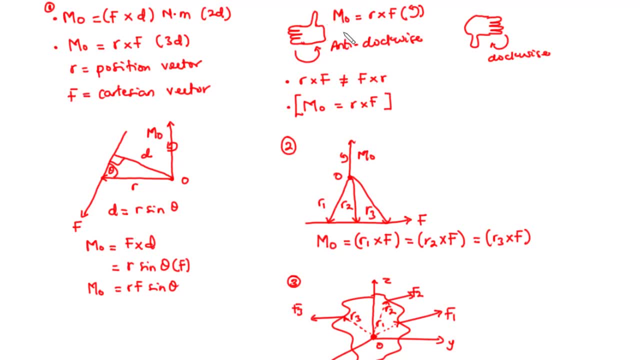 So, depending on where the thumb is facing, you can either have a clockwise moment or an anticlockwise moment. So moment is not always anticlockwise. It could be clockwise or anticlockwise. Now, based on what we've studied so far, 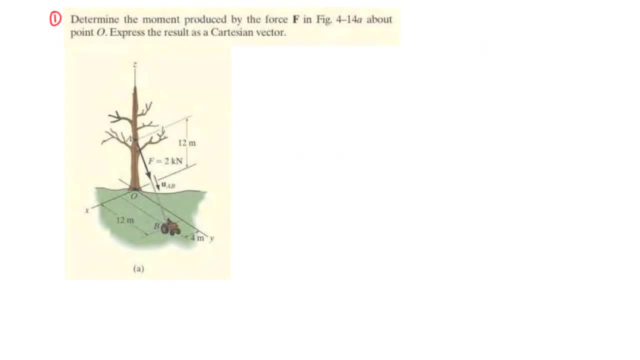 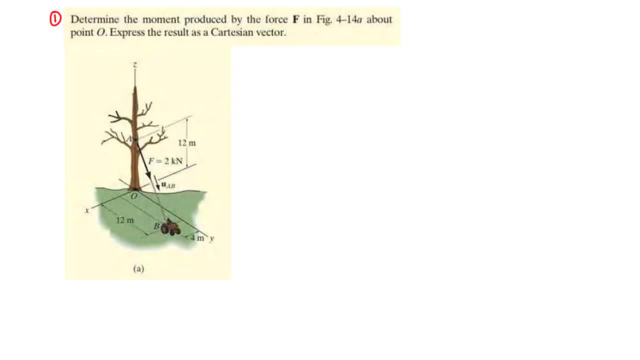 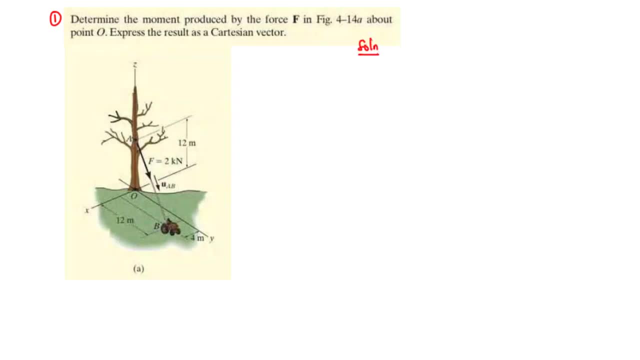 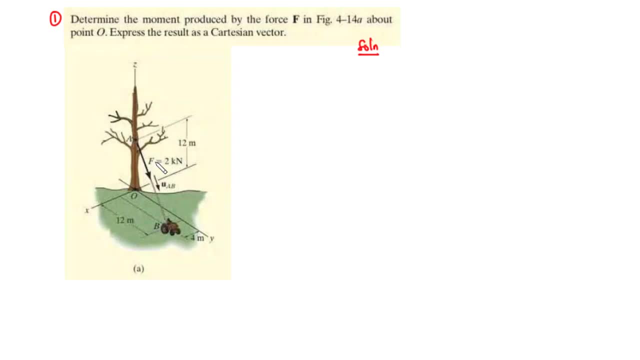 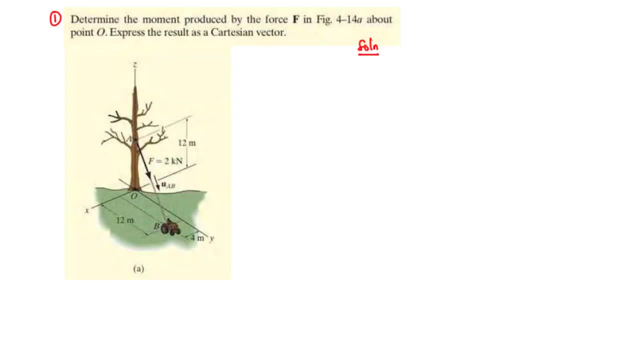 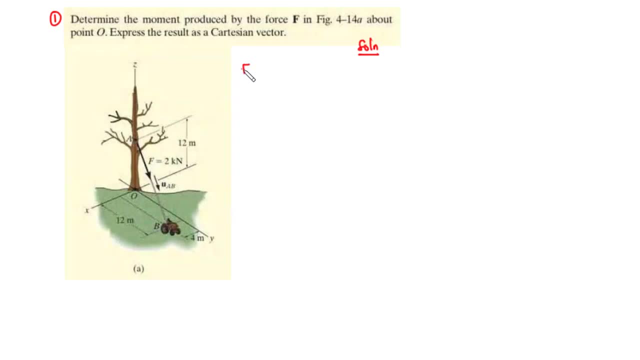 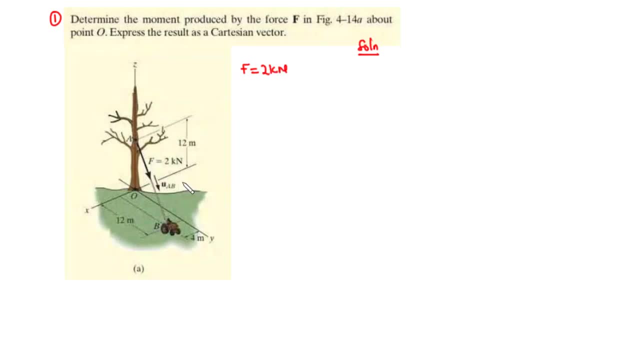 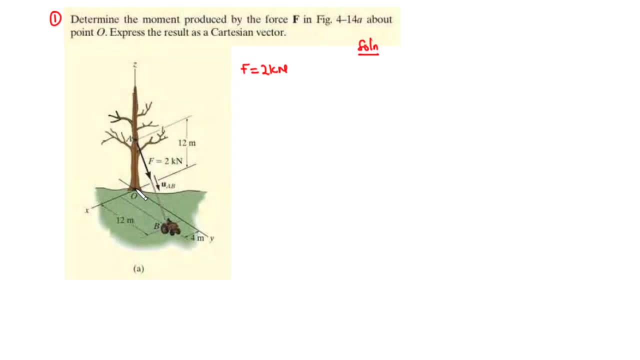 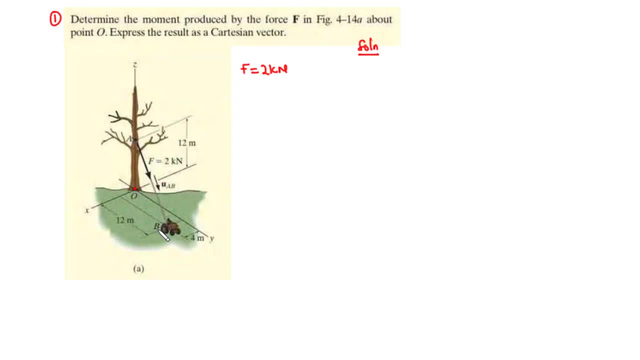 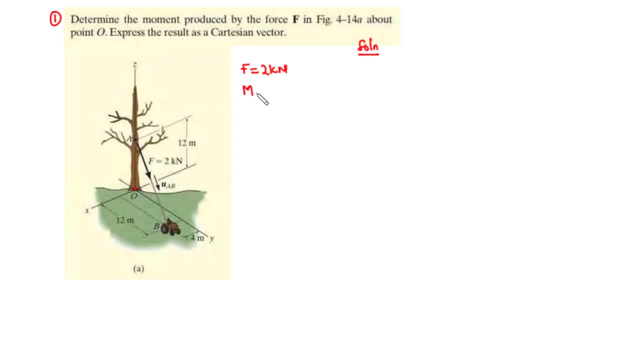 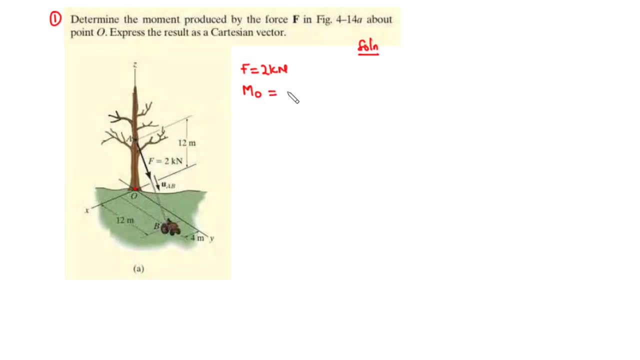 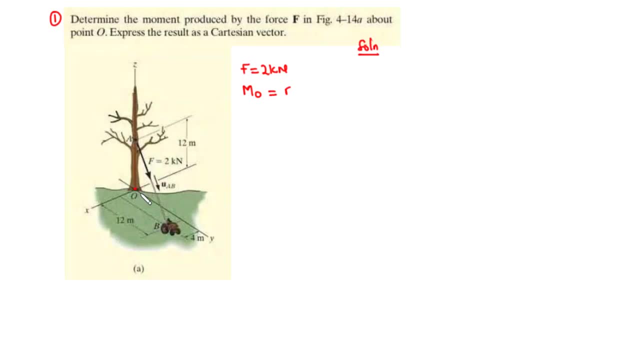 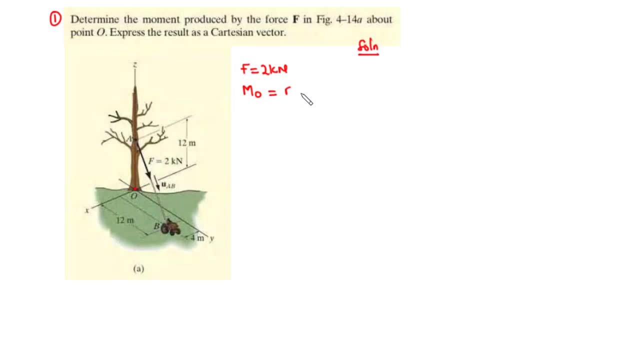 Determine the moment produced by the force F in the figure 4F on the line of action of F and the force F represented as a Cartesian vector. Now, in this case, we are given the force F to be 2kN, hence we need to represent the force. 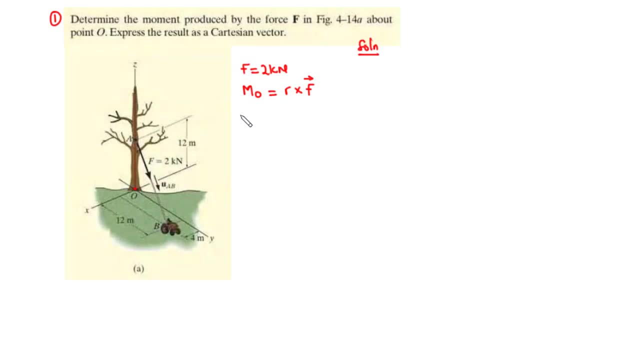 F as a Cartesian vector and that is given by the product of the magnitude of the force and the unit vector directed along the line of action of the force. Now we know the magnitude of F. however, we don't know the unit vector UAB. So let's try to find the unit vector UAB. 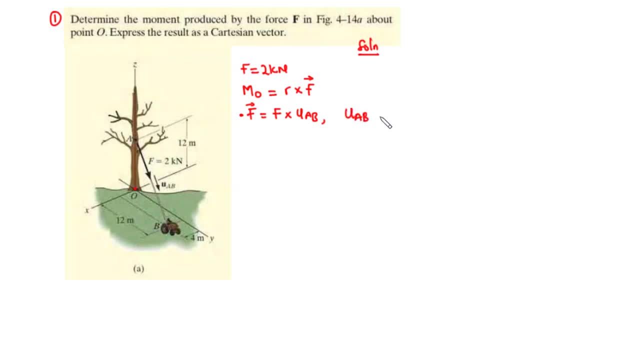 So the unit vector UAB is given as Now. to find the unit vector UAB. we are going to move from point A to point B Now to find the unit vector UAB. we are going to move from point A to point B Now to find the unit vector UAB. we are going to move from point A to point B. 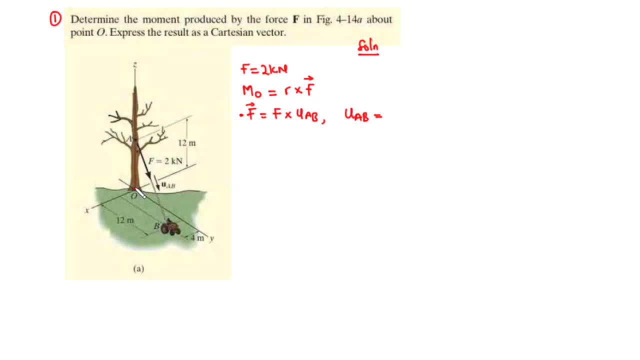 Now, whenever you move from any point towards point O, then that is a negative value. You are going to obtain a negative value, and the moment you move from point O to any point, then you have a positive value. So, basically, that is the information that you need to obtain. 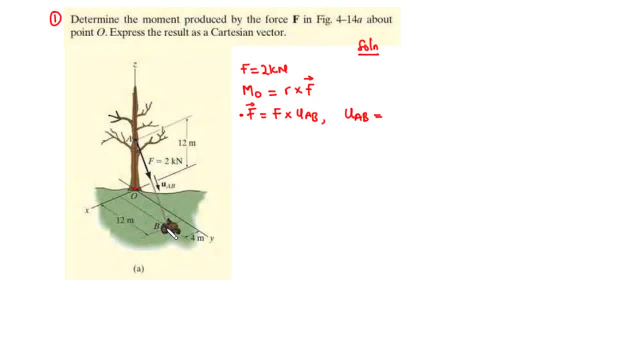 And so to move from point A to point B, it means that you are going to move along the X, Y, Z axis. So first along the Z axis, you move from point A to point O. Now, since you are approaching point O, it means that you have a negative value. 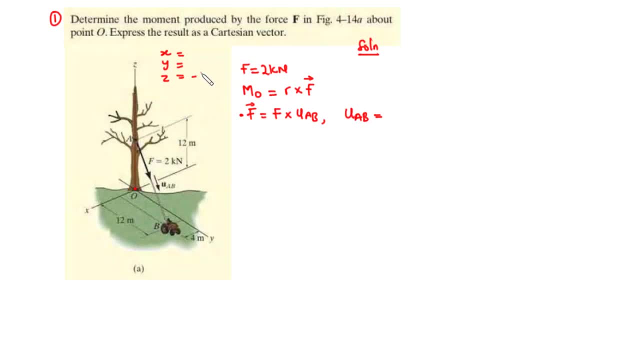 So that becomes negative 12.. So negative 12K in meters. And then you need to move along the X axis. So away from point O means that you have a positive value which is 4 meters. So that is 4I, also in meters. 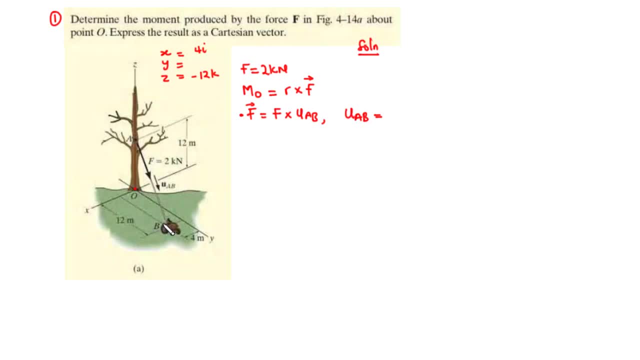 And then you need to move away from point O along the Y axis, and that is also 12 meters, So you have 12J. Therefore, the unit vector UAB is equal to 4I plus 12J, minus 12K, all divided by the square. 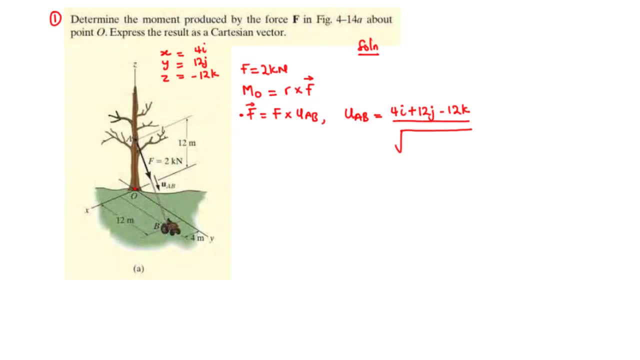 root of 4I, The sum of the squares of their coefficients. So you have 4 square plus 12 square plus negative 12 square. Now this is equal to 4I plus 12J minus 12K, all divided by: 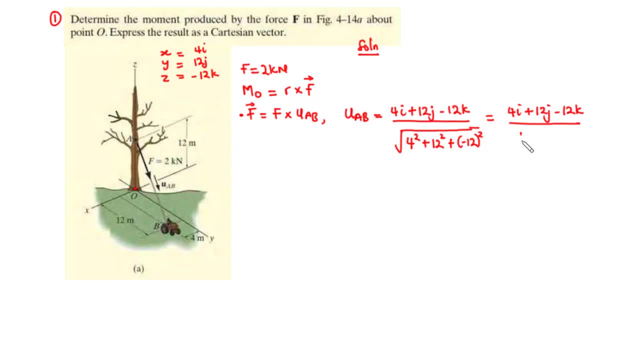 Now, when you simplify this, you are going to get 17.5.. Okay, 17.4356.. So when you solve this, the denominator, you obtain 17.4356.. Now let's further simplify. We have UAB to be equal to 4 divided by 17.4356 gives 0.2294, plus 12 divided by 17.4356 gives 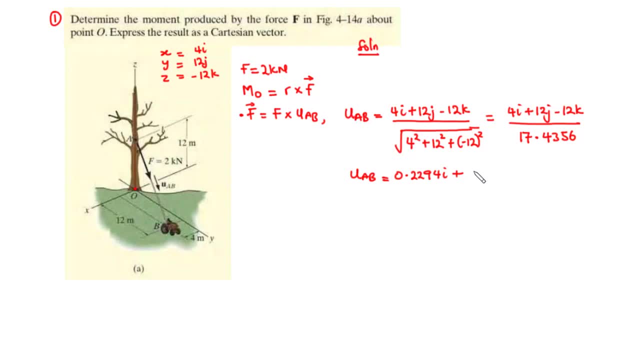 0.2294.. Okay, Okay, Okay, Okay. So we have 0.6882J and then minus, we have the same value, 0.6882, and then K. So this is the unit vector UAB, That is, the unit vector in the direction of the force. 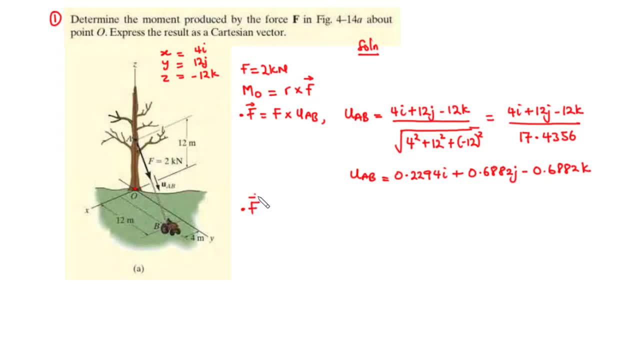 Now let's move on to find the force as a Cartesian vector. So that is equal to. We have the magnitude of the force 2K. Okay, Okay, Okay, Okay, Okay. Now we have 0.03 Snow Newtons times UAB. so times 0.2294I plus 0.6882J minus 0.6882K. 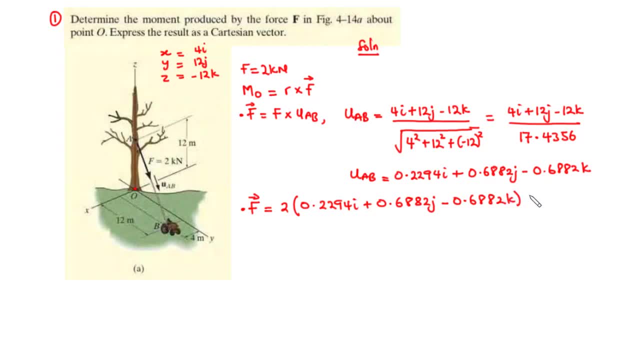 Okay, Okay, Okay. So you multiply 2 across and then you have 0.4588i plus 2 times this, you have 1.3764j minus 1.3764k, And this is in kilonewtons. So after finding the force F, or representing the force F as a Cartesian vector, 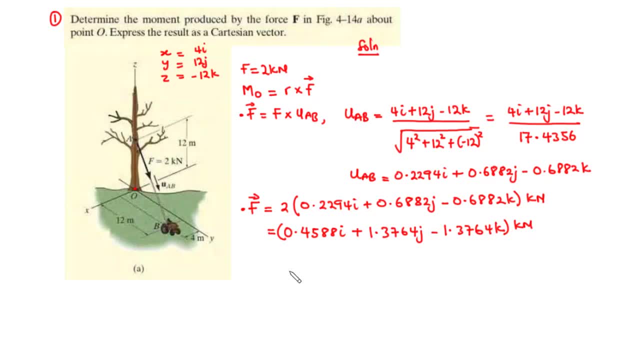 We are left with the position vector. Now, according to the principle of transmissibility, To find the moment about a point. If you have more than one position vector, Then any of the position vectors directed from O To any point in the position vector On the line of action of the force. 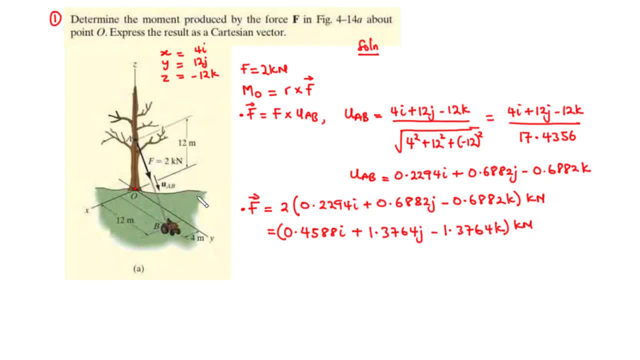 Produces the same moment. Now in this question We can specify two position vectors, So one, we have position vector from O to A, So that is RA. And then secondly, we can also specify a position vector From O to B, And that is called RB, So we can use the cross product of either RA and then F. 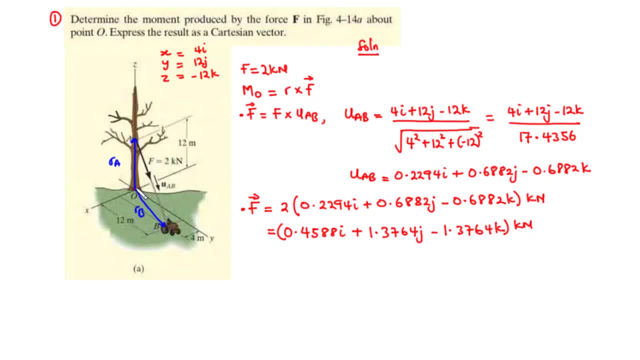 Or RB and then F. Since the position vectors are directed from O To any point in the line of action of F, It means that we are going to obtain the same value. So lets move on As we find the position vectors: RA and then RB. So for RA. 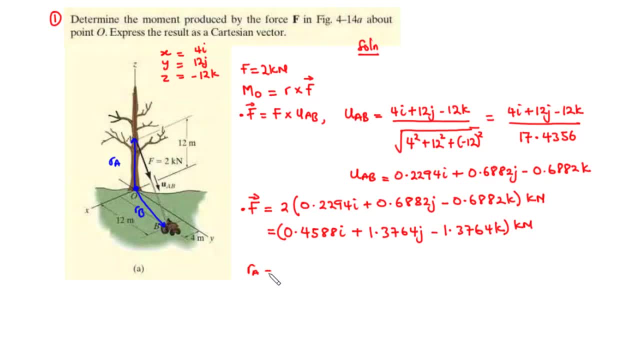 for r? a. we are going to move from point o to a, and since we are moving away from o, it means that we are going to obtain a positive value. so we have 12 k. so that is 12 k in meters. so we have 12k in meters. 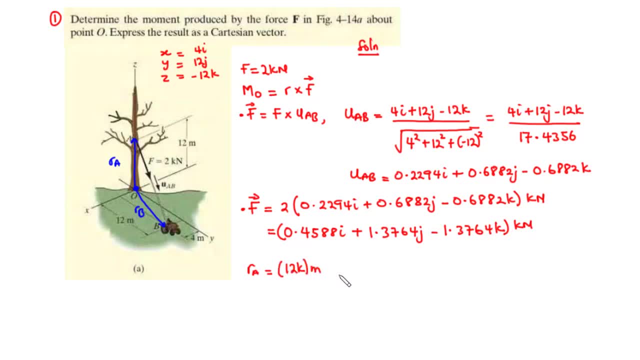 and then for rb, we are going to move from point o to b, so first we need to move along the x-axis, that is four meters, and then along the y-axis, that is 12 meters. in all cases, we moved away from point o, which means that we are going to obtain a positive value. so we have. 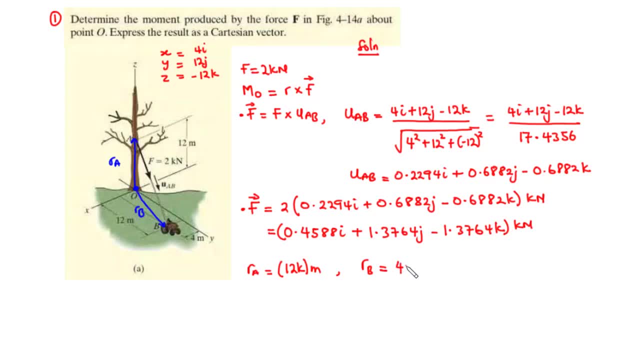 four, 4i plus 12j, And notice that this is in meters. Now, looking at the two values, You realize that RA looks more simpler, And so, for the sake of this example, We are going to consider the moment to be The cross product of RA and then F. 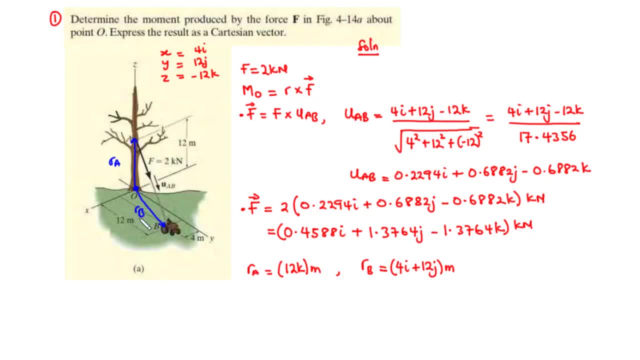 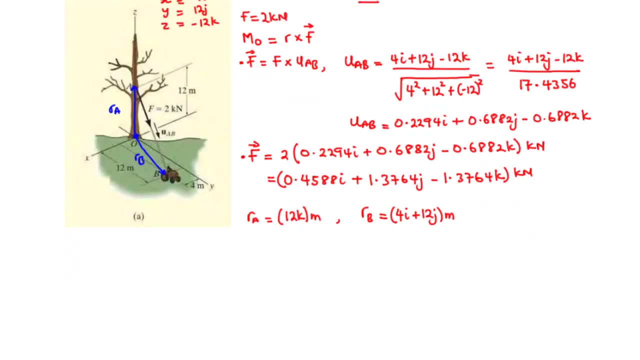 Now you can as well consider the cross product of RB and then F, And you realize that you are going to obtain the same value of moment. So let's try to find the moment of this force about the point O, And so we have the moment MO To be equal to the cross product of RA and F. 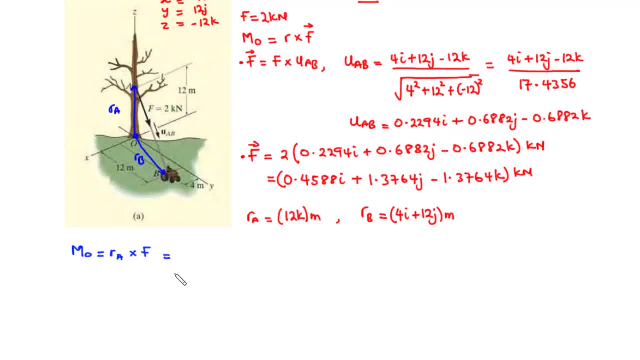 And to find the moment, We are going to construct a determinant, And we are going to construct a determinant And we are going to construct a determinant That is a 3x3 determinant, Where we have the first rule To be the unit vectors i, j and then k. 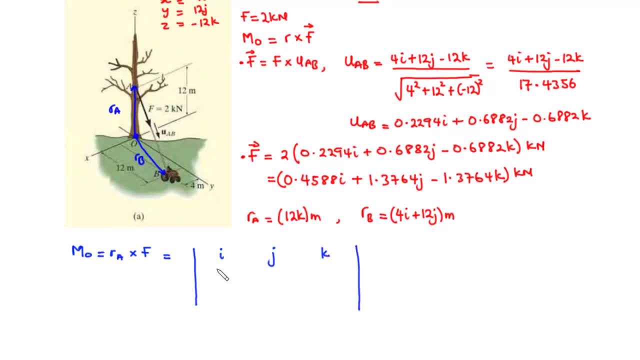 And then for the second rule, We have the coefficient of RA. So for RA we have 12k, Which means that The x component is 0, Y component is also 0, And then we have the z component to be 12, Also for the force vector. 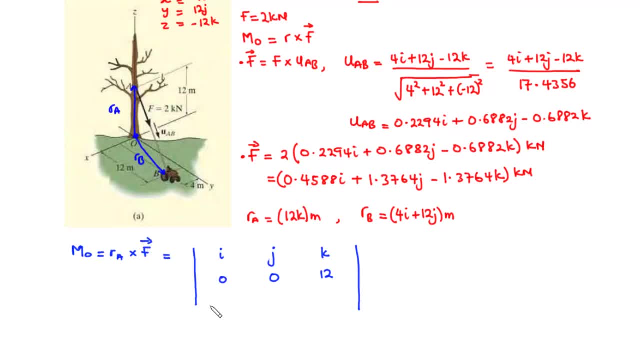 We have the x component to be 0.4588, Y component 1.3764. Z component negative: 1.3764. Now let's try to find the determinant of this 3x3 matrix. And that happens to be the moment of the force. 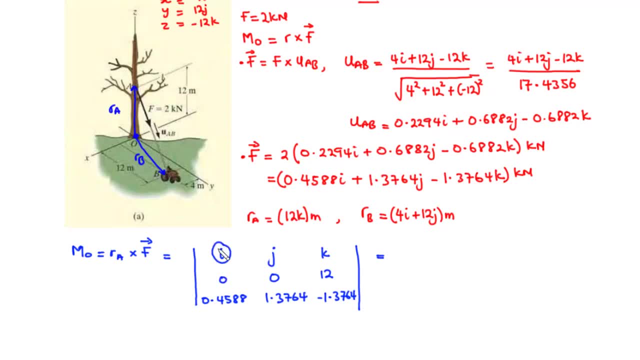 So first of all We select i, And then we cross the row And then the column containing i, And so we will be left with 0, 12, 1.3764, negative 1.3764. So we are going to have i on the outside. 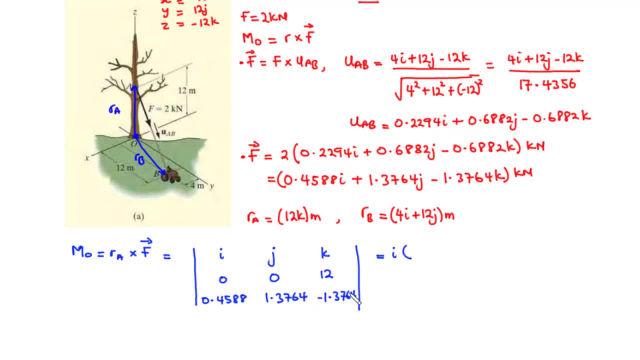 So that is positive i And then into brackets. we have This value times 0, It becomes 0 Minus 1.3764. times 12 gives 16.5168 And then minus j. So for the determinant it's always plus, minus plus. 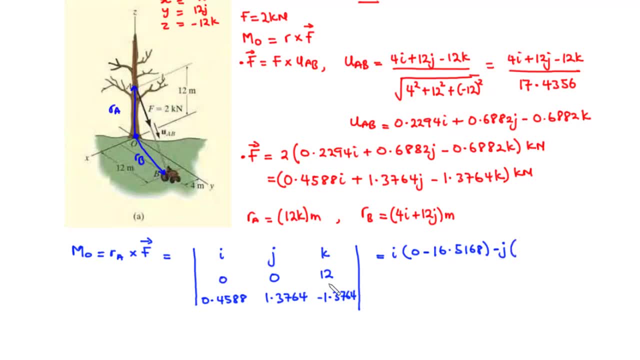 So minus j Into brackets, We select j And then we cancel the row And the column containing j, And so we are left with 0, 12, 0.4588, and then negative 1.3764. so we multiply this value by zero and that is still zero minus. 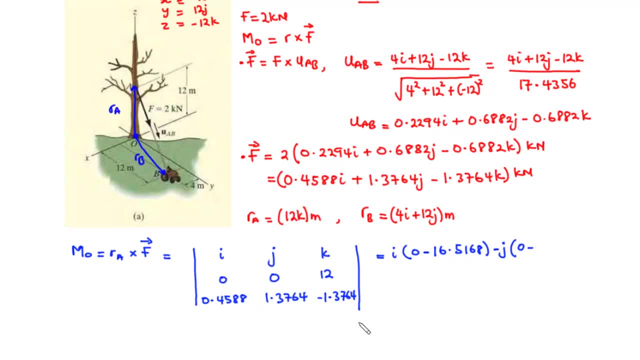 we multiply 0.4588 by 12 and then we obtain 5.5056 plus k. also. we select k, we cancel the row and column containing k and then we multiply this value by 0, that is, 0 minus this value, also by 0, 0, and so we are going to simplify so we have i times negative of this that becomes negative. 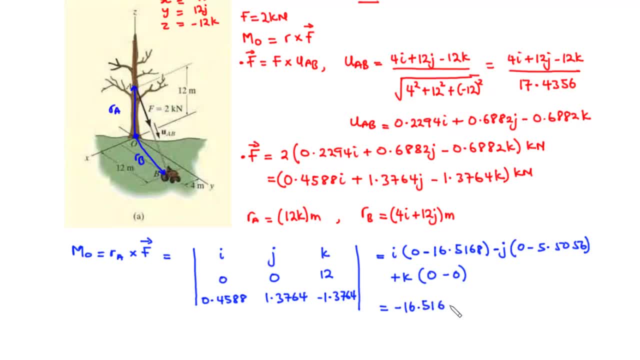 16.5168 i, and then we have negative times, negative, so that becomes positive. so positive: 5.5056 j, and then plus 0 k. so plus 0 k. we can choose to leave that out, and so in actual sense we can further simplify this as negative: 16.5 i. 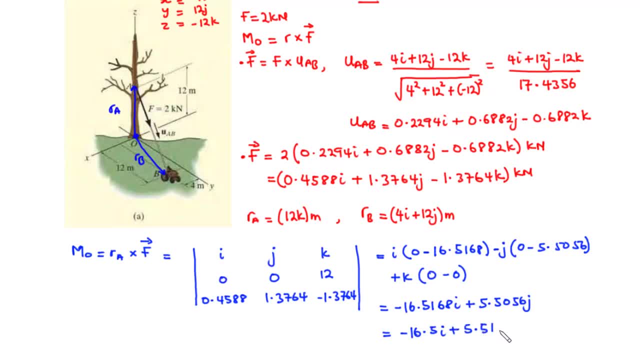 plus 4k, 5.51 g, and notice that this is in kilo newtons meter. so that's it for today's video. thanks for watching and see you in my next video. in the next video on moment of a force, we are going to solve two more examples. bye, bye.